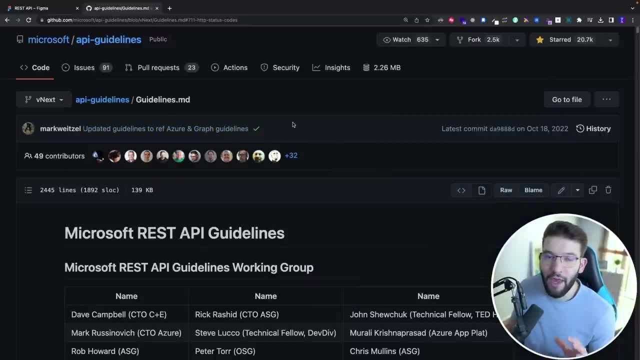 tell you that these guidelines and the advice you're going to see in this video are heavily inspired by the Microsoft API guidelines. So if you go to GitHub in here, Microsoft has a REST API guidelines for their internal team and for other public team. They are published in GitHub and you 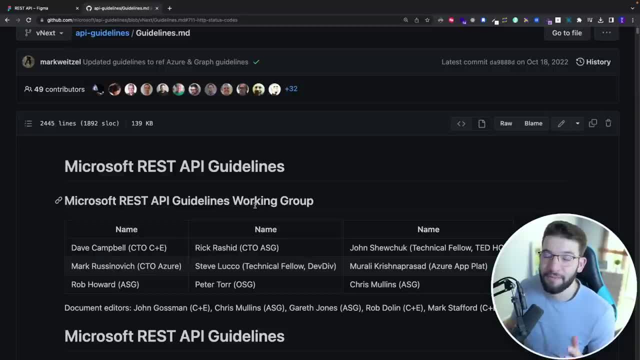 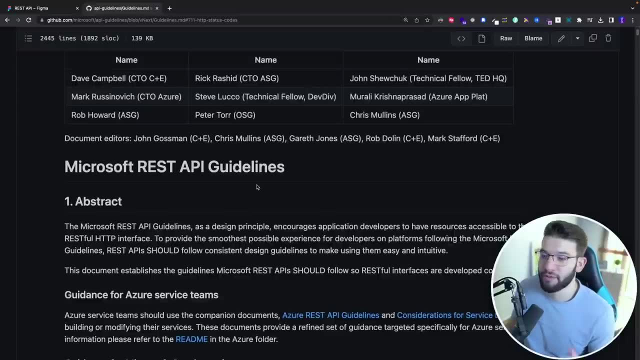 can use them, and those guidelines are very specifically made for REST APIs. They're pretty good. They have a lot, a lot of stuff. So I really advise you guys to go ahead and like re-through it out this and actually understand everything that's going on here and reason behind. 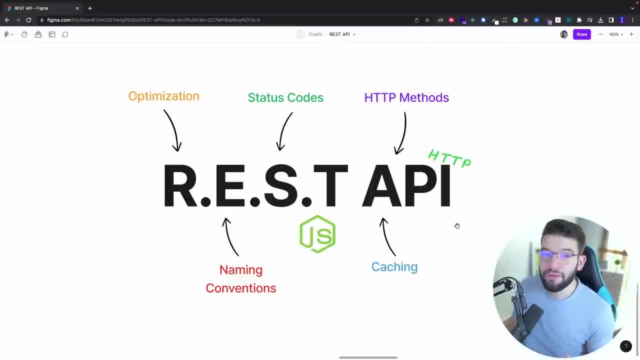 So these are the five mistakes that you're probably doing wrong in whenever you're trying to actually make or write your own RESTful APIs, and what are the best advices to completely avoid those? So, starting with naming conventions- So naming your APIs is a really, really big deal. 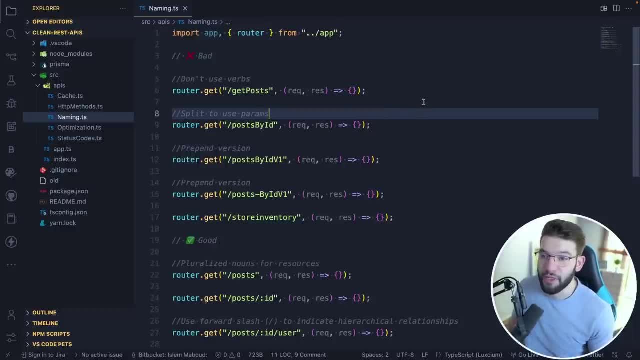 Either actually makes your APIs look simpler and easier to read, either for your team, who maintains the code, or for consumers, who are going to be using the API at the end. So, for example, in here for a bad practice. for example, you don't want to use verbs on the API endpoints itself, For example. 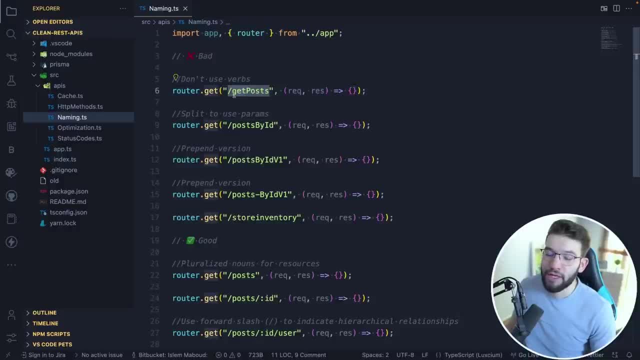 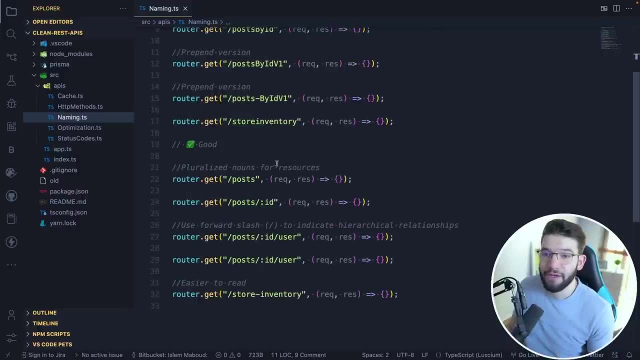 in here when you try to git post. you don't do git post Here. you're using a kind of a verb and you're just, like you know, concatenating that with the name. You don't want to do that. You only want to use proper names and the name should be pluralized. So it could be something like: 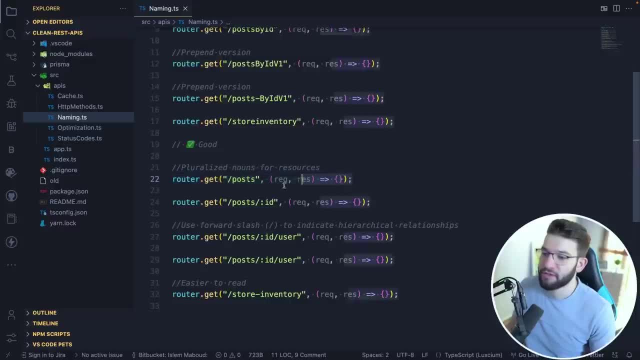 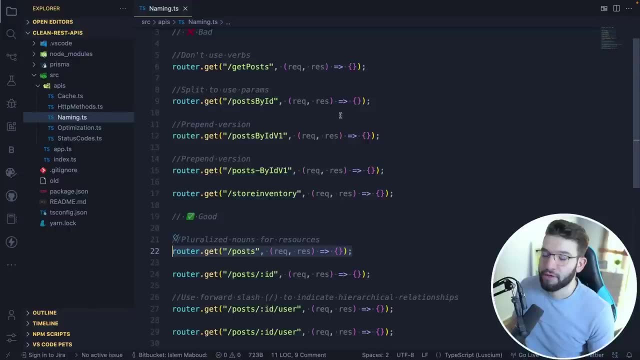 post and that's it. You just do forward slash. this is the endpoint and this simply insinuates that: oh, this API is going to return all the arrays and posts that are in the database, For example, instead of doing post by id, which is a very complicated name and it makes it super hard. 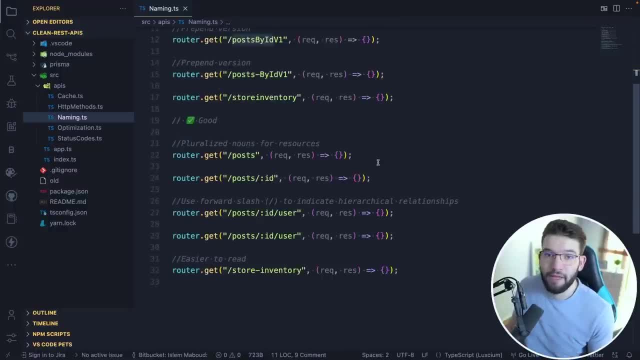 to do that, you want to use parameters, and this is actually the main thing why RESTful APIs set those parameters this way. So you do post and you make sure there's still a plural when you provide an id, So like a forward slash, and there's actually the parameter id that tells it: oh, 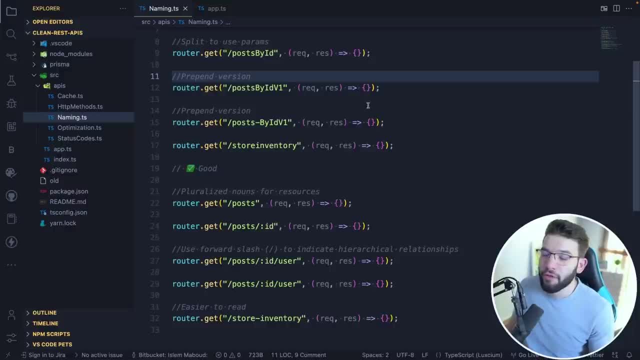 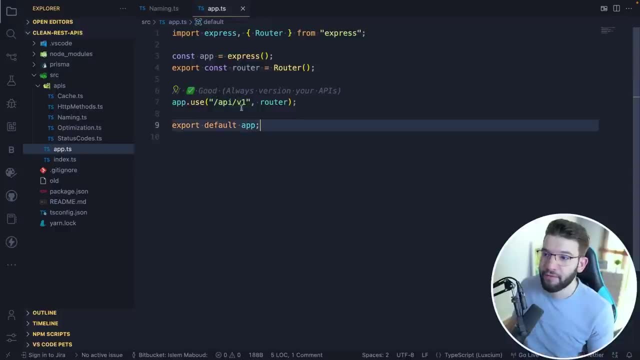 I want to find a post by this particular id. Another wrong thing in here is adding v1, or versioning, at the end of the endpoint. Instead of doing that, you should actually put your code in the prepend, the v1, for example, in here. this is the router and when we do the api, so it's actually. 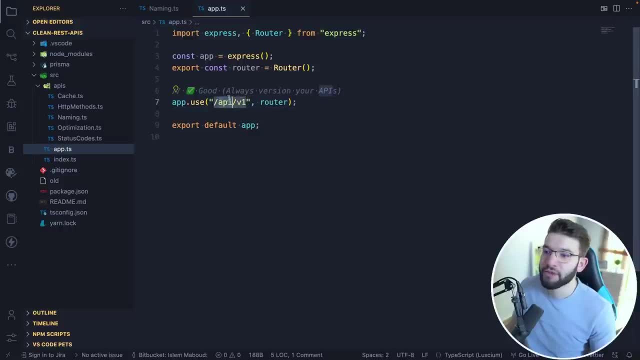 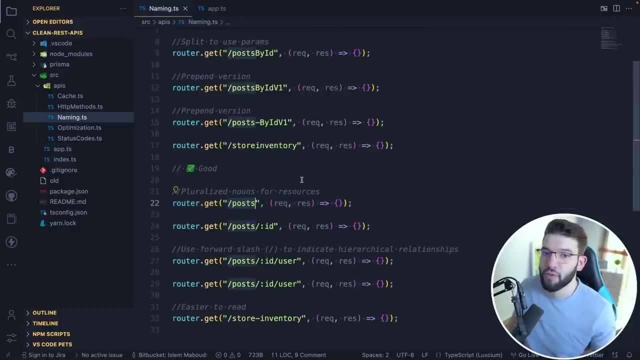 the. you know we're just like pre-pending this one, so it goes like: api: forward slash v1. then it comes to this, for example: forward slash post. so it's always pre-pended. whenever you want to add another version, it's very easy for you to add that v2 and v3 and so on. if it's something like this, you don't. 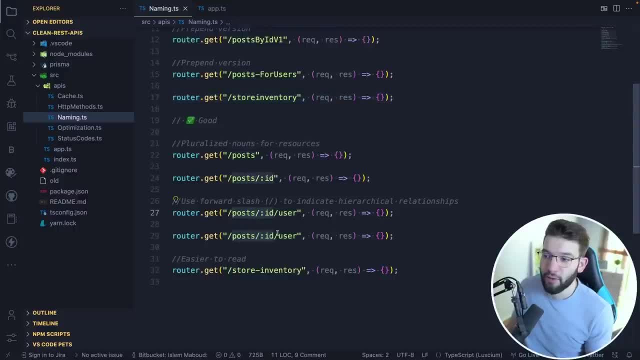 want to do that either. you just want to do like, for example, post: you want to find a post by id and user in here is taking away, so you're going to return the user for that particular post. so the forward slash in here always indicates the hierarchical relationship between the different. 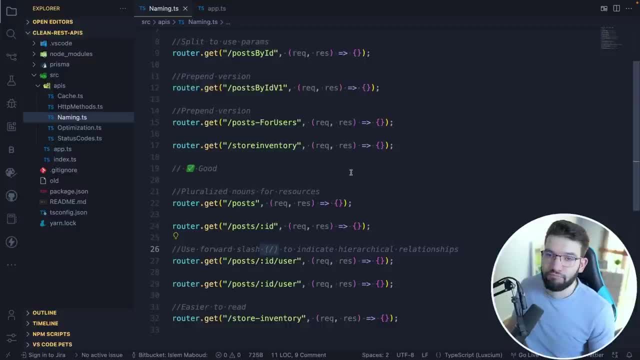 entities you're actually exposing throughout your api and, for example, you've got like a complicated name like this one where it's store inventory. you can't actually use capital letters in an actual api or a url, because this is going to end up in the url eventually. so what else you 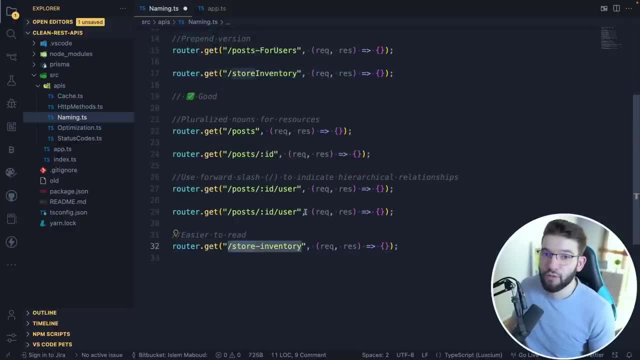 can do is actually use a hyphen or a dash in here, so this will make the api a little bit more readable and easier to tell exactly what this one is going on instead of just leaving it like this. so it's going to be a little bit more readable and easier to tell exactly what this. 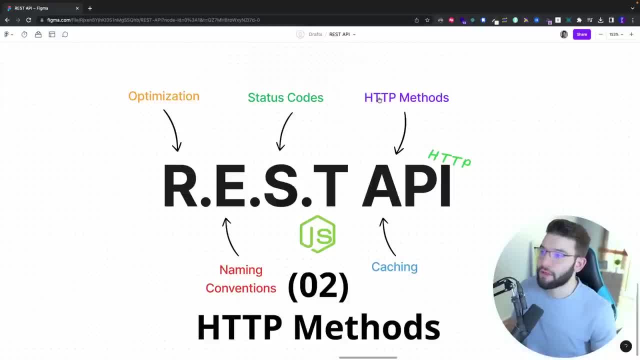 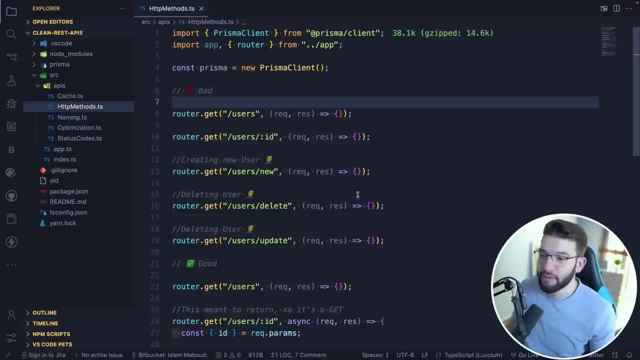 one is going on instead of just leaving it like this. so this will make the api a little bit more, or just even with the lowercase thing. the second most important thing are http methods. so if you don't know already, http methods are put there to insinuate and actually differentiate between. 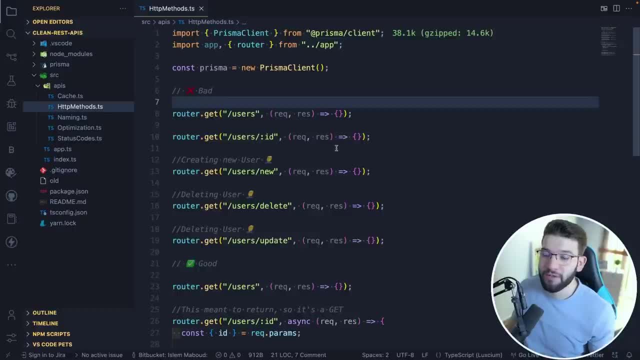 what each operation is going to do and what each endpoint is going to accept, and do so, for example, in here, instead of using a git method for all of your stuff in here and actually only changing the endpoint. for example, here you're fetching users, that's fine. you're fetching users by id, that's. 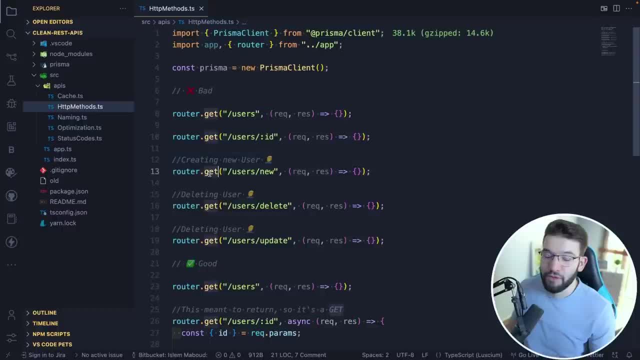 fine. here you're actually adding or creating a new user, but you're still using a get request. that doesn't make sense. or either maybe you're deleting or updating, you're still using gets and you just like adding this to the endpoint. no, that's a very bad approach. 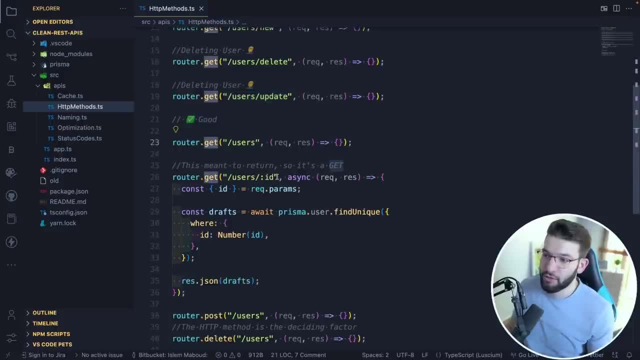 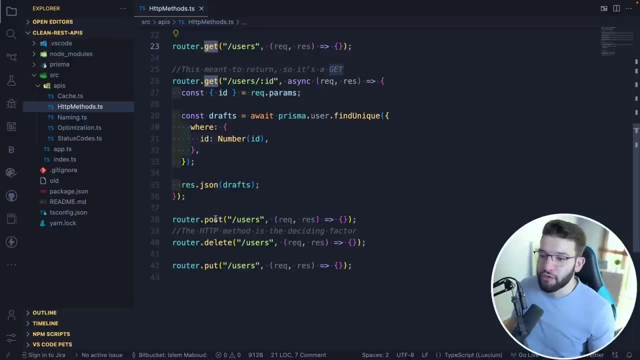 one study would do for getting here, obviously, just when i just do get in here. as simple as that. but for all those stuff you want to use the appropriate http method for it. so for example, in here for creating your user, you want to use post for deleting an actual user. when i use 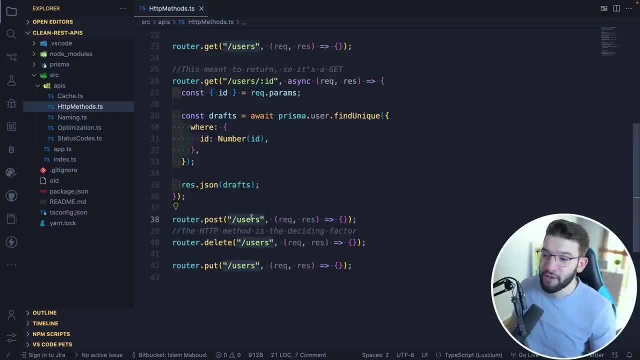 deletes, and all the endpoints in here are actually the same. so the only thing that differentiates between those apis and those handlers is actually the http method. so if you use the http method itself, so use, like, for example, post for creating delete method for deleting an actual user. actually you're going to provide the id and stuff like that and put in here. 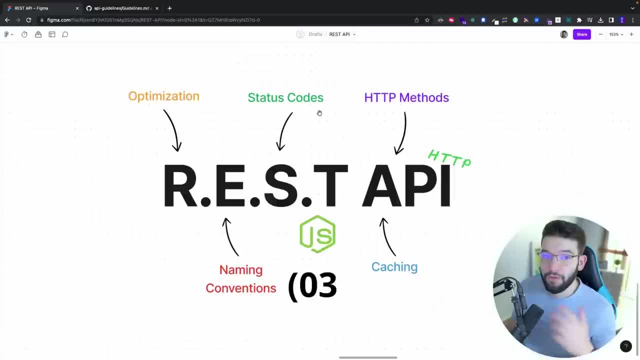 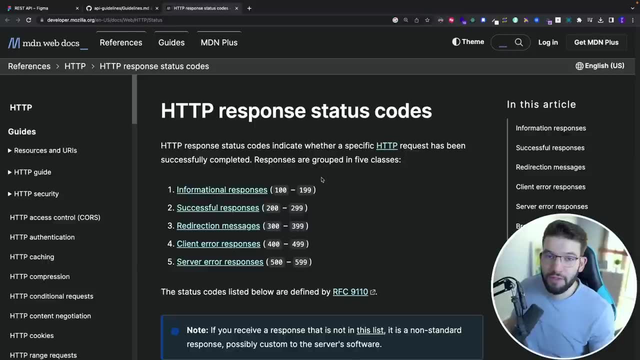 for updating a particular already existing user. for the third one, it's the status codes. so, for example, if you go to the mdn real quickly in here, you're going to know that there is a bunch of status codes, http status codes, and each range of status code is actually for a specific reason. so 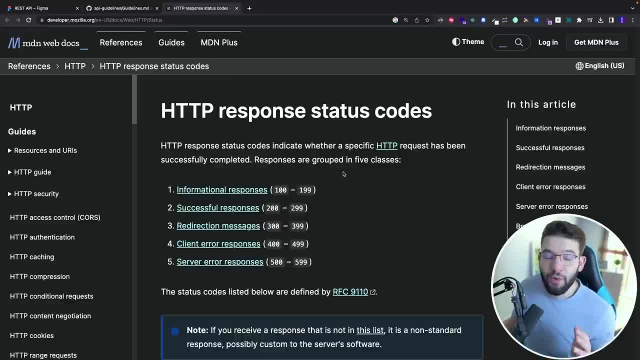 depending on your response from the server. you need to use the appropriate status code for the browser to know exactly what's happening, and you're going to need to use the appropriate status code for the end user for like a cdn or a cache you're using in the middle or anything else that will. 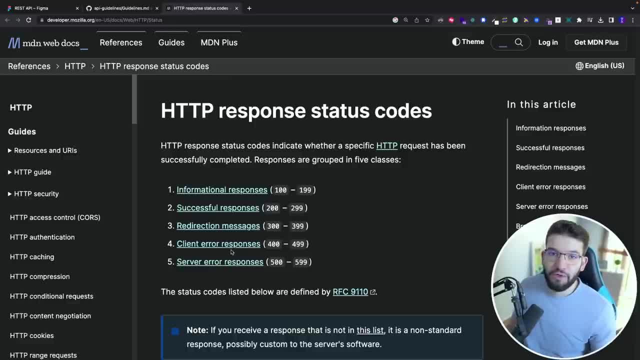 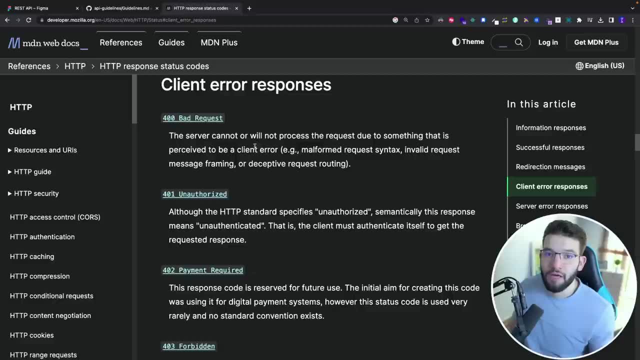 make it work the perfect way it should be. so, for example, in here for client error responses, in here there's like 400 for a bad request that insinuates: oh, the client sent me a bad request that you should revise the payload and the payload that i just sent me is not accepted at all. or maybe like: oh, 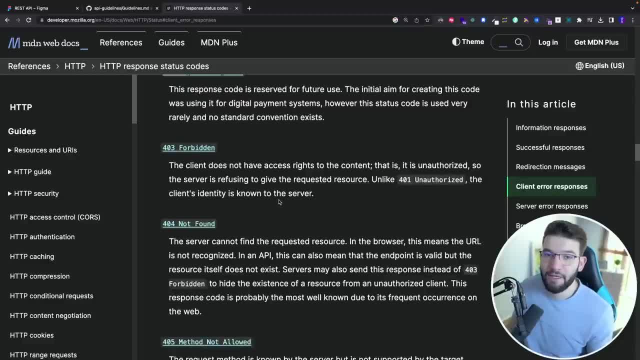 404 from a not found resource for a not found entity in the database, or something like that. so, for example, in here- what a lot of developers actually do- let's say, oh, you got a handler in here that actually does a lot of work for you. so, for example, in here you're going to need to 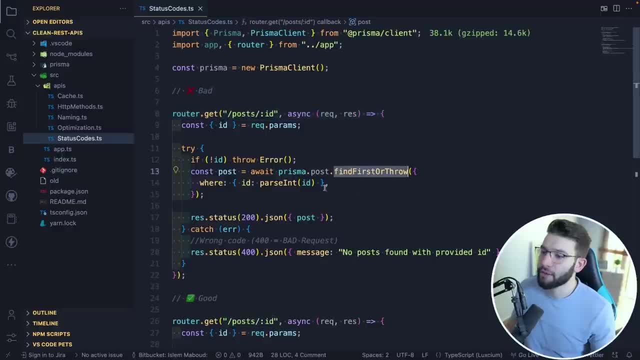 actually fetch you a post by id. so you go and look into the database in here using the post id and stuff like that. if you find it, you're going to return. oh, status 200, that's completely fine, because you're just returning and you turn the actual post, that's good. but if you don't find this, 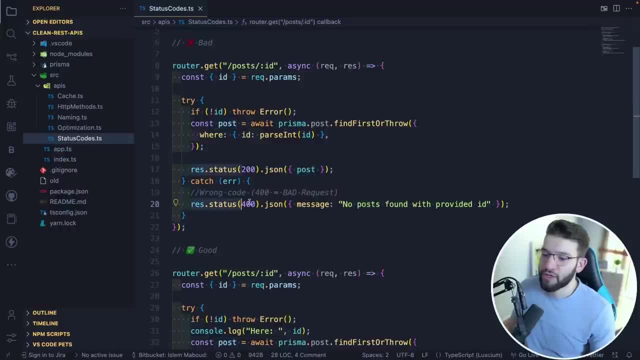 one, you go: oh wrong, or yeah, i'm going to do a status 400 and remember a 400 is for, like, a bad request that tells you: oh user sent a bad request. but in this case it's not exactly a bad request because the user sent an id and if the id doesn't exist in the database it's not a bad request. 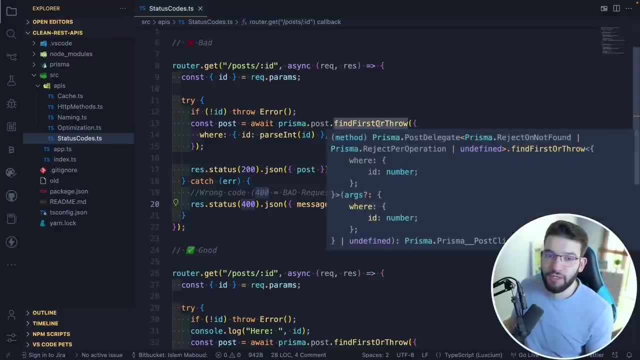 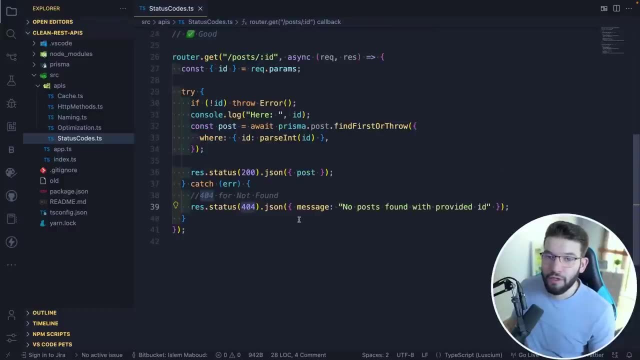 it's in the database. it's not a fault of the actual user. the user is still sending a right piece of data. so instead of between 400 in here we should return a 404 for not found. so 404 in here would work perfectly with a message: no post found with provided id. so, for example, if we go to 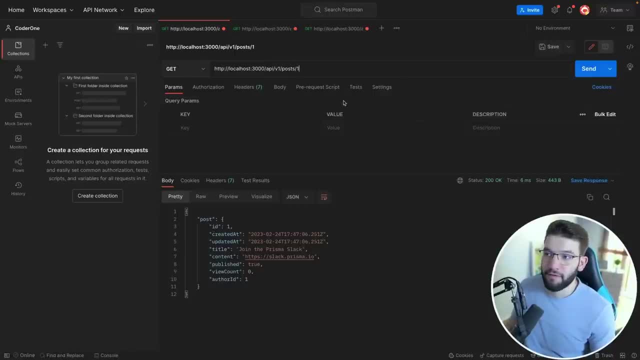 postman in here. i do request with with id one. that's good he found this one, for, for example, if i use zero, which is not found, i still get status code 400- bad request, and if you change that to 404, i do another request in here. there you go now. instead it's returning a bad request. 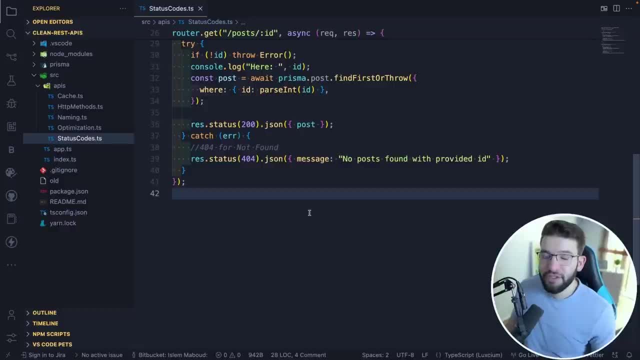 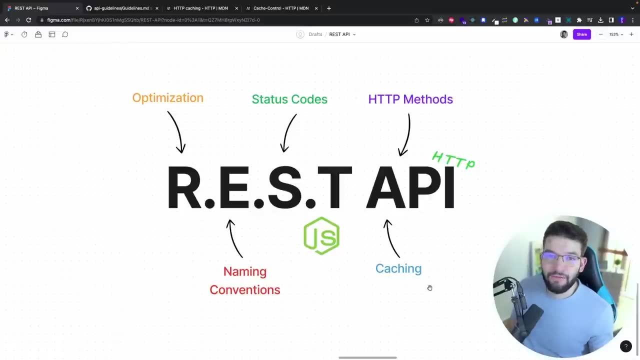 it returns 404 for not found, and that's so perfect. and this actually applies to all the other status codes, from 500- internal error- into 200 and so on and so forth. the fourth thing that i see a lot of developers actually completely ignoring, especially newbie developers, is caching. so if 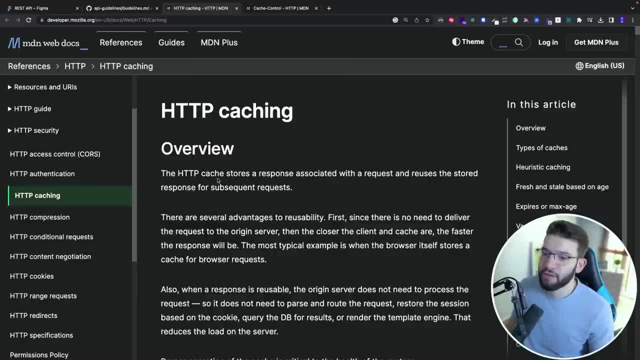 you look at the http caching topic in the mdn documentation, you're going to know: oh, the http cache stores a response associated with a request and reuse it- the stored response from subsequent requests. so that simply means when you actually do a request that basically looks like the previous request all the users are doing and you have, like cash, valid cash either in. 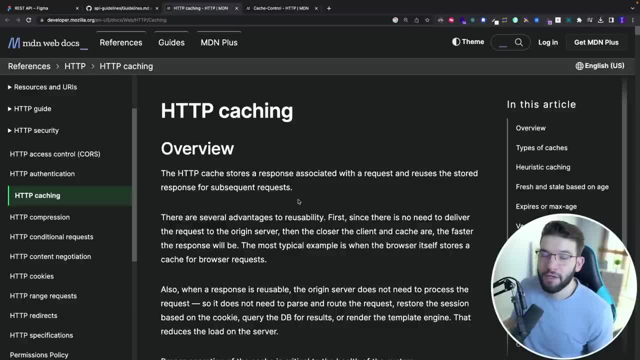 the cdn or the browser itself. the server won't need to make a new response. the response is just going to be retrieved from the cache and the server is not going to be reached out anyway. and that going to make our servers work so much better. it's going to serve more people. 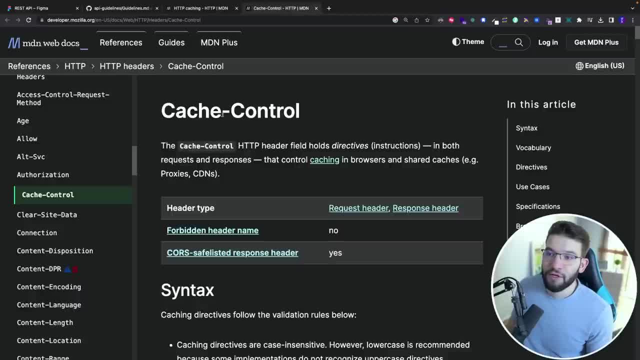 and it's going to save us a lot of coasting time- and this is all done through the cache control header, which is a header that sends back to the browser and the cdn or whatever from the server itself, depending on the type of request and the response. 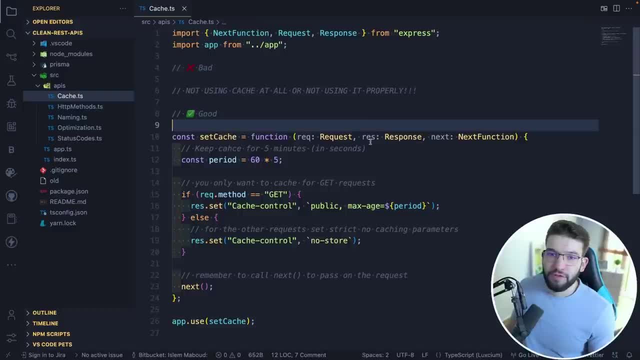 is actually sending to tell it whether to cache or not. so for example, here in caching for a bad usage is not using cache at all or not using it properly. now for a good approach. this is just an example for the current use case i'm having, which is just a blog that serves post and post can be. 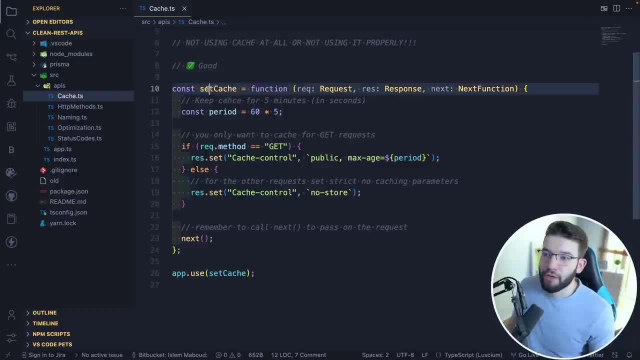 like published, like per day or something. so, for example, here you do a middleware, a middleware called set cache. that's going to say simply request response and next an express middleware, and here we got a period. period is actually in like seconds, 60 times five to get five minutes. 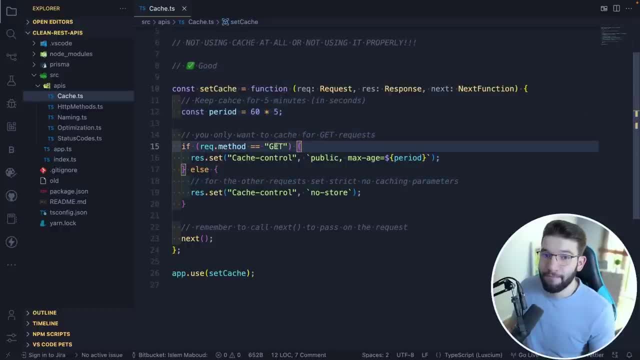 in seconds and we simply do a quick check-in. so if it's a git method, which is what you should cache most of the times, you're gonna send back the cache control header to be public, because that could be cash pretty much by anyone, and you put the max age in here to be five minutes. 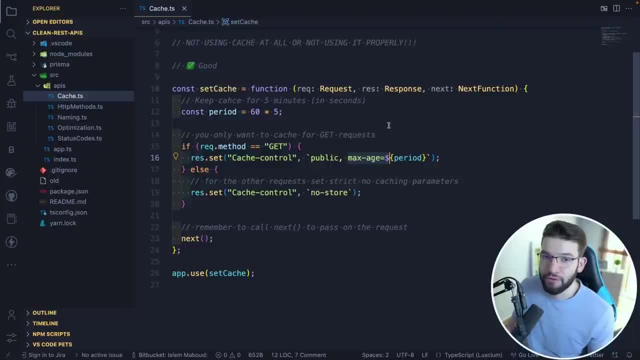 so everything in here is going to be cached for five minutes in the browser or in the cdn? if it's not, if it's like post, puts or any other type of request, i don't want to catch that especially. you want to like, you don't want to cache puts or post or delete stuff, so cache. 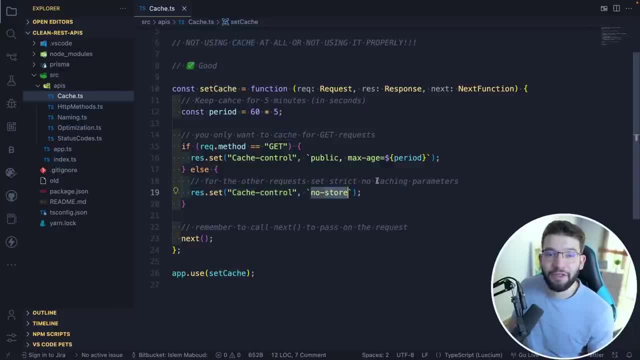 control in here should always be no store, but yet again, this should depend on your type of application. if you have a different type of location, the cache strategy and how you handle in cache should be different. and simply in here: last one is just called next and we use that set. 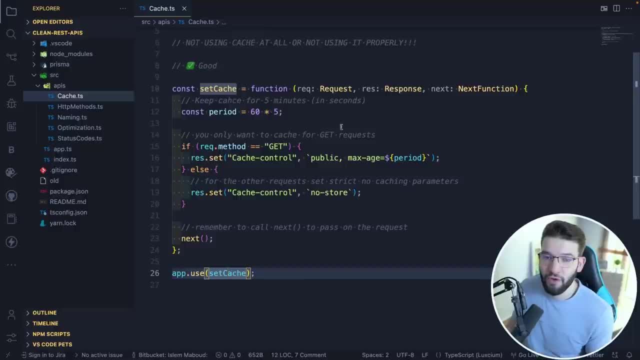 cache middleware. so express is going to use that for every single time a new request is going to make to the server, and if it's git request, i'm just going to catch that out, and this is going to make it super, super fast for us. so i really advise you guys to make sure that you're not 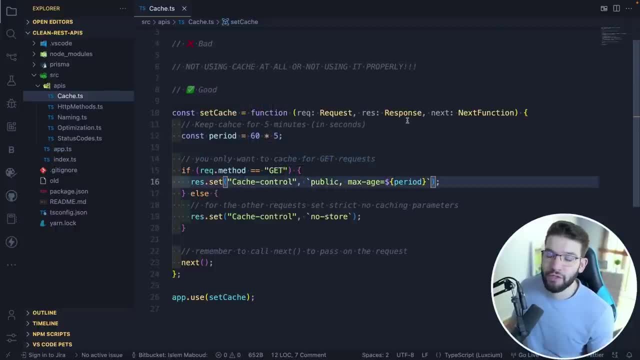 going to have to do that, and then you can just go ahead and check how caching works and how the cache control header actually works and all the stuff that goes inside of it to make it better, to make your apis, to make your apis more reliable and faster. and last thing in here is optimization. 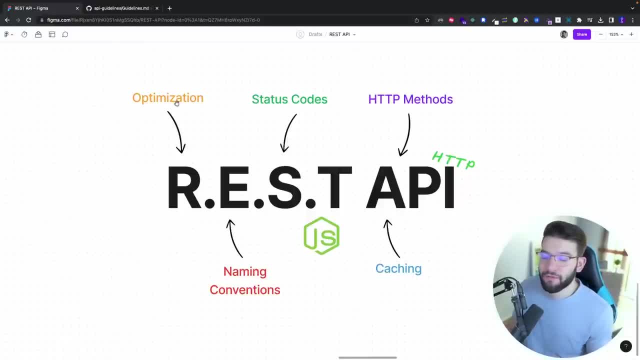 and there's actually quite a lot of stuff that goes inside of the optimization topic for restful apis in general, but one of the most important parts is trying to reduce the number of http requests, or restful api requests, for getting a single piece of data, that is. 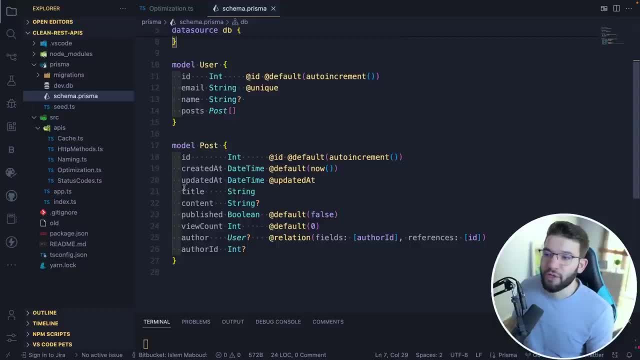 related together. let me show you what i mean. so in our database in here what we got, i've got an user and we've got a post and each post in here has an author and the author in here is going to be like an user, so it has a relation with the user in here and the relation is going to be saved. and 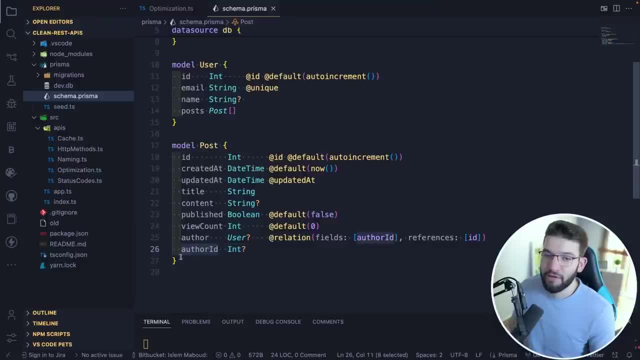 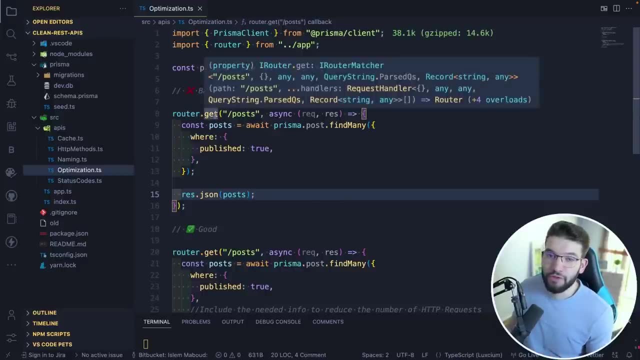 the author id. so the user id is going to be saved in the author id. so simply, each post will have one author. now let's say we've got an api in here where the user is simply going to get like a post and array of posts. so we're going to display or a post in home page or something like that. so we're 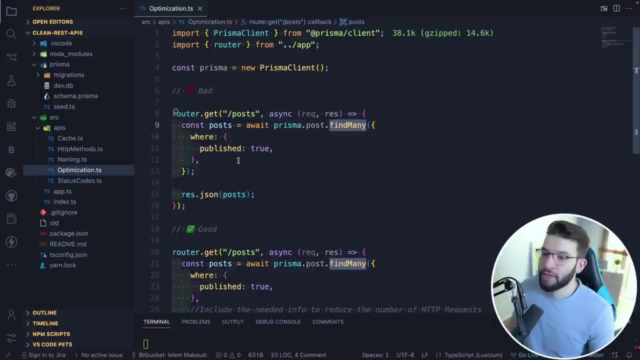 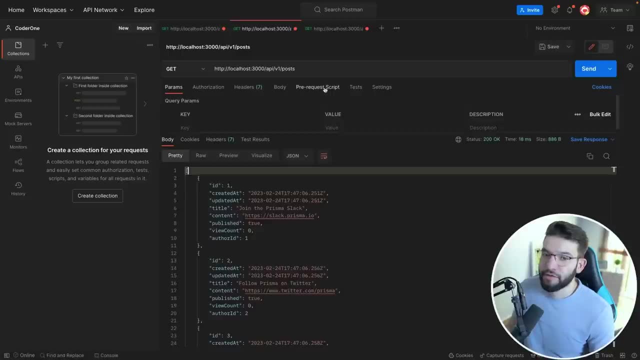 in search page. so what we're doing in here? oh, we find post, we do find many- and we say, oh, if it's published, you're going to return that, and simply we're returning posts. but this is not very well optimized. so if we go to our postman in here and try to test the api by sending a request, getting 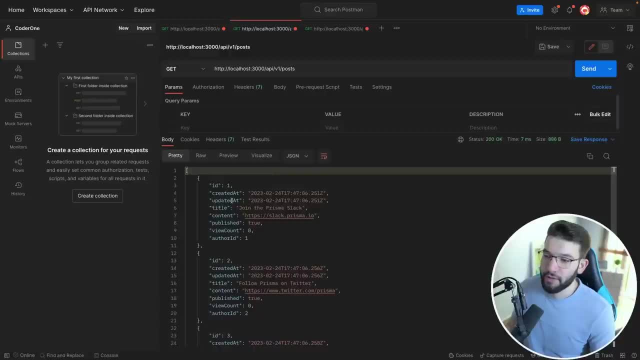 a post. we return three posts in here which are in the database as close in here. it doesn't return the author but instead it returns the author id. so when we try to display the post in our home page or application, mobile application or anything, when we try to do that and try to display the